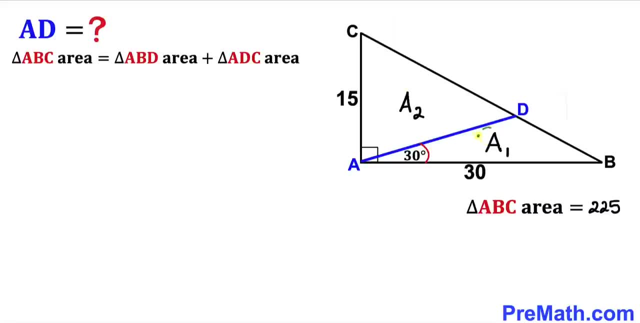 triangle ABC is going to be the sum of these two individual areas, a sub 1 plus a sub 2.. Therefore, this equation can be written as area of this triangle ABC is going to be a sub 1 plus a sub 2.. But we know from this equation area of this triangle ABC is a 225.. So therefore, I'm going to 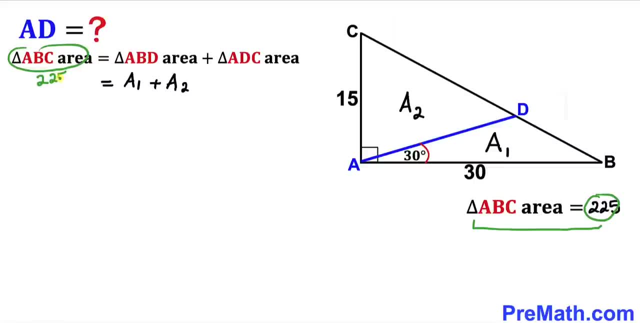 replace this one by 225.. So, therefore, this equation is going to become 225, equal to afraid, one plus a sub 2. and now we are going to calculate these areas: a sub 1 and a sub 2. and now, since we are interested in finding the length of this side ad, let me go ahead and represent this side. 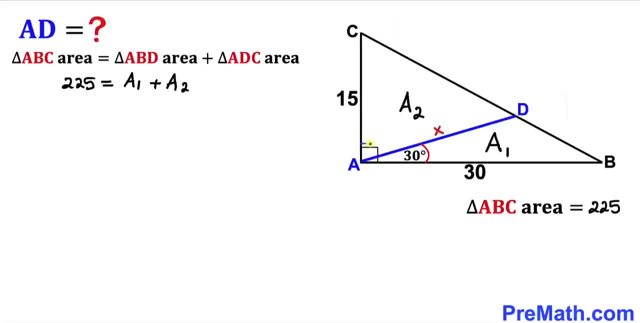 by x units. moreover, we know that this angle is 90 degrees and this angle d ab is 30 degrees. so therefore, this angle d? ac is going to be 90 minus 30 is going to give us 60 degrees. now here's our next step. let's go ahead and calculate the area of this triangle: a, b, d, which is a sub 1, and. 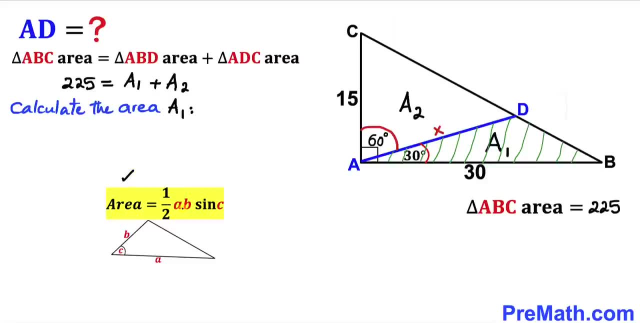 now let's recall the area of a triangle formula. area equals to a half times a, b times the sine of c. as you can see in this triangle, a and b are our side lengths and c is the angle of the triangle and b is the angle of the triangle and c is the angle of the triangle. 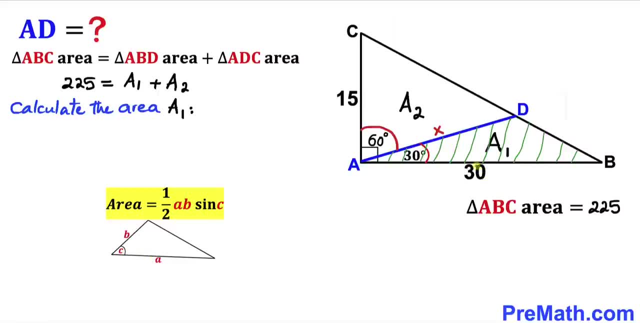 between these two sides and in our case our side, lengths are 30 and X and the angle between them is 30 degrees. so, therefore, our area is of one is going to be a half times 30 times X, times sine of 30 degrees. and here's our next step. 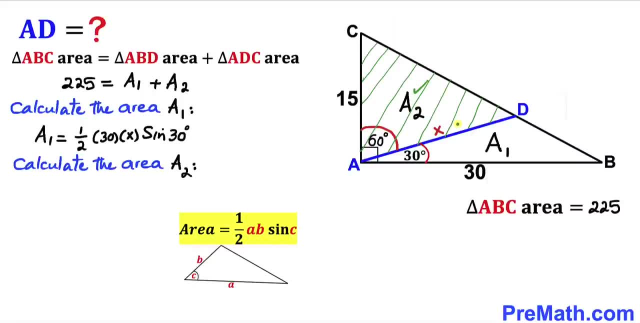 let's go ahead and calculate: the area is of two of this triangle adc, and once again we're gonna be using this area formula. in our case, our sidelines are x and 15 and the angle between them is 60 degrees, so therefore our area is of two. 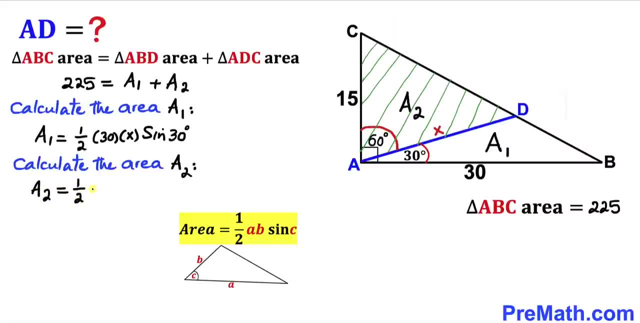 is going to be a half times x times 15 sine of 60 degrees. and here we figured out our a sub 1 and a sub 2 values. let's go ahead and plug it in in this equation. therefore, our. this equation could be written as 225 equal to. i'm going to replace a. 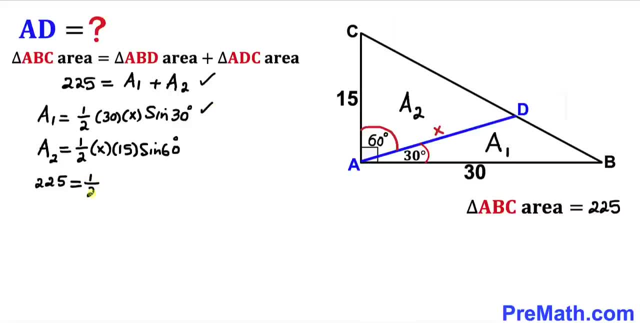 sub 1 by this right hand side, which is a half times 30 times x, sine of 30 degrees plus i'm going to add this one as well. so that's going to be. i have times x times 15, sign of 60 degrees, and 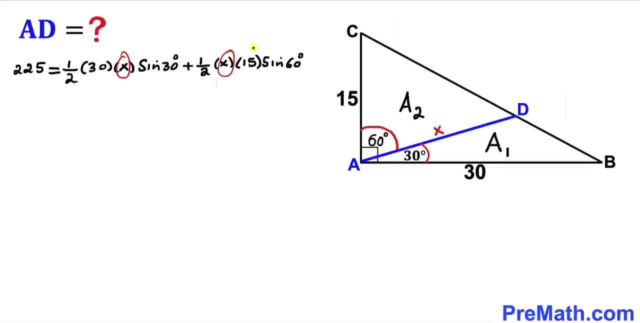 now we are going to solve this equation for x, and now let me show you how to find this sign of 30 degrees and sine of 60 degrees in an easy way, without using a calculator. now let's focus on this 30, 60, 90 special right triangle, and we know that this 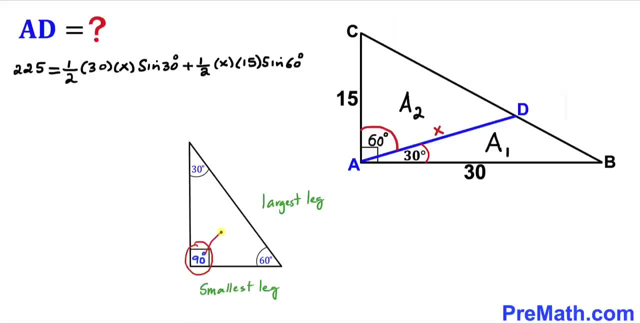 9 resolution is 0.. Georg and 6 are work keeps. Then let's estimate the distance of dimension. The lastolution of dimension is 0.. Georg and 6 are Work keeps. 90 degrees is our largest angle. So the side opposite to this one is going to be. 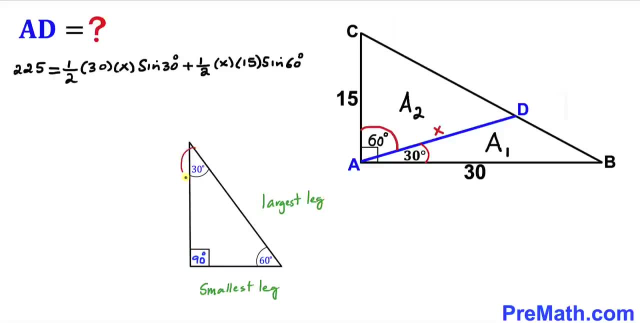 this side is going to be longest leg And this 30 degrees is our smallest angle. So the side opposite to that one is going to be our smallest leg. So in such kind of triangle this longest leg is twice this smallest leg, If this smallest leg is one. 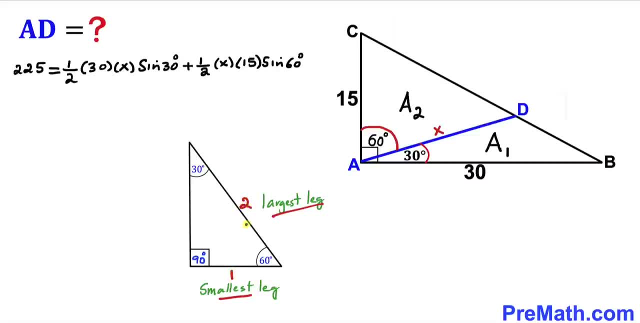 then this largest leg is gonna be two times That one is going to be two units, And if we use the Pythagorean Theorem, this, our third leg, is going to be square root of 3.. Now, let's recall this: SOHCAHTOA, We are going. 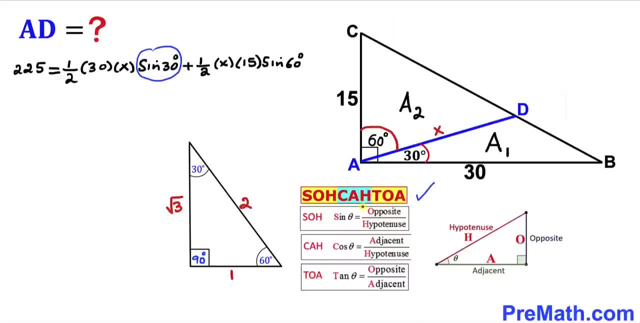 to find the value of sine of 30.. So, therefore, we are going to use this sine of theta equals to opposite over hypotenuse And, in our case, for angle 30 degrees, this side is our opposite and this side is our hypotenuse. So, therefore, sine of 30 degrees is going to be simply: 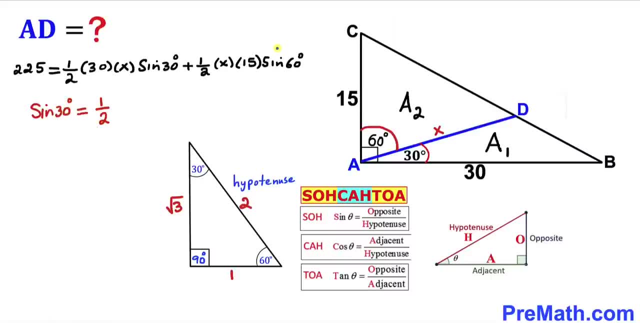 it's going to be 1 divided by 2.. And now we are going to calculate this sine of 60 degrees for this angle. 60 degrees, This side is our opposite and this is our hypotenuse. So, therefore, sine of 60 degrees is going to be opposite. in our case, is square root of 3 divided by 2.. So therefore, I'm 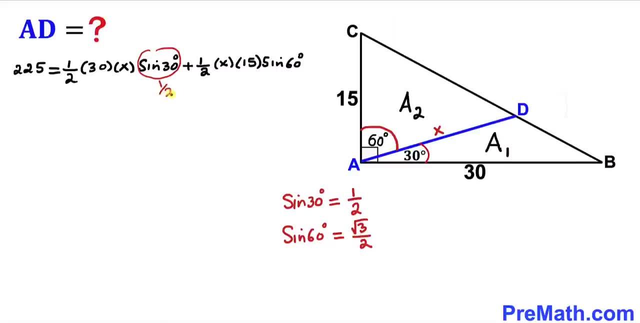 going to replace this sine of 30 degrees by 1 divided by 2, and sine of 60 degrees. I'm going to replace it by square root of 3 divided by 2.. As you can see in this next step. Now let's go ahead and simplify. 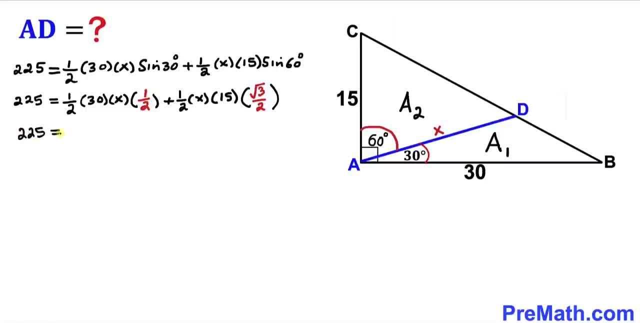 this thing that is going to give us 225 equals to, and that is going to give us 30 x divided by 4. plus, that is going to give us 15 times square root of 3 times x divided by 4.. And here on the 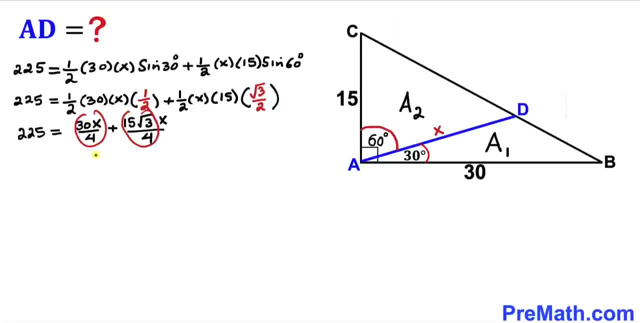 right hand side, we can see that between these two terms, 15 divided by 4, is in common. So this is going to give us 15 times square root of 3 divided by 4.. And here, on the right hand side, we can see that between these two terms, 15 divided by 4, is in common. So this is going to give us: 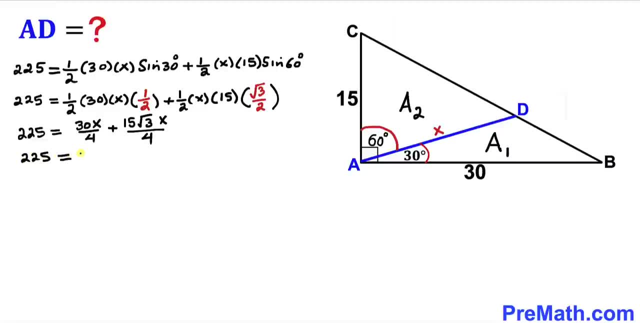 therefore, I can write this thing: 225 equals to 15 divided by 4 outside. So we ended up with the 2x plus square root of 3 times x. And now let's go ahead and multiply both sides by the reciprocal of this one, which is 4 divided by 15 on this side and 4 divided by 15 on this side as well. 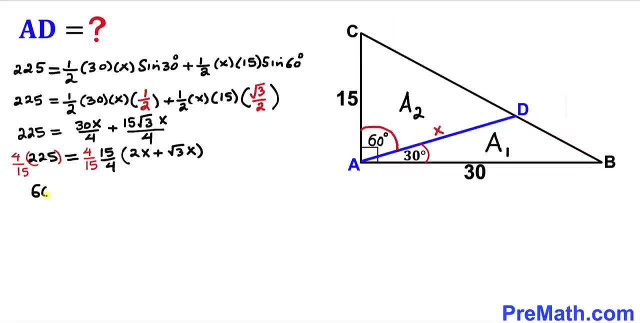 And on the left hand side, when we multiply this thing, that's going to give us 60 equal to. these are cancelled out, And here we can factor out x times. this is going to give us 2 plus square root of 3.. And now let's go ahead and divide both sides by 2 plus square root of 3.. 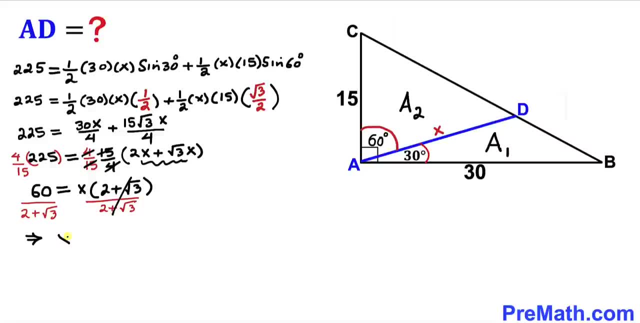 This is gone. So, therefore, our this x value turns out to be 60 divided by 2 plus square root of 3.. And now we know that this x represents the length, ad. So therefore ad turns out to be equal to 60 divided by 2 plus square root of 3.. 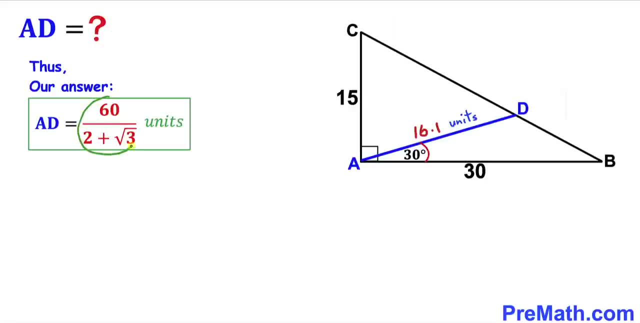 So thus our ad length turns out to be 60 divided by 2, plus square root of 3 units, And that is approximately equal to 16.1 units. Thanks for watching and please don't forget to subscribe to my channel for more exciting videos. Bye.